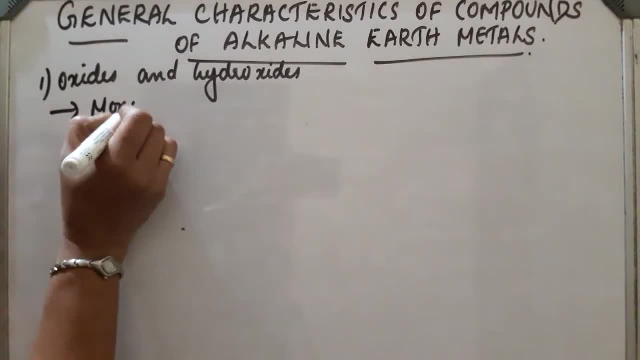 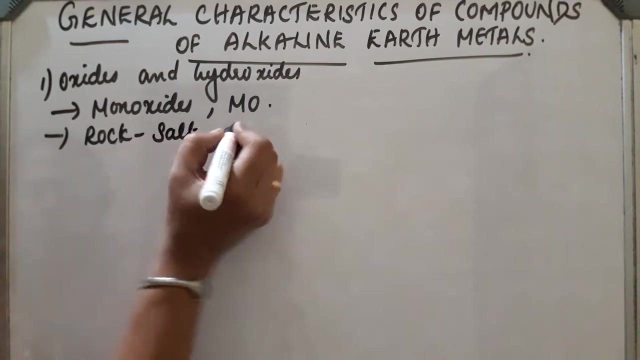 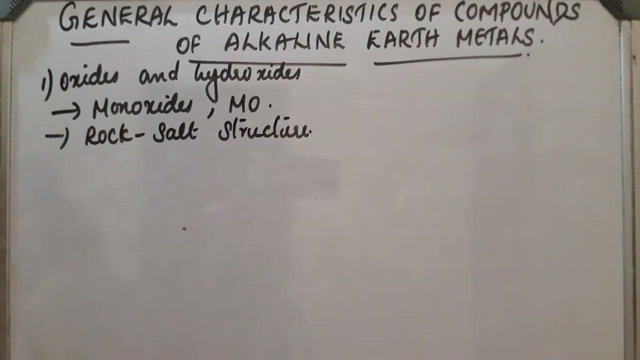 and form monoxides. they form monoxides, mo okay. and except beryllium oxide, all are having rock salt structure. rock salt structure- okay. and beryllium oxide is covalent in nature. beryllium oxide is covalent okay. 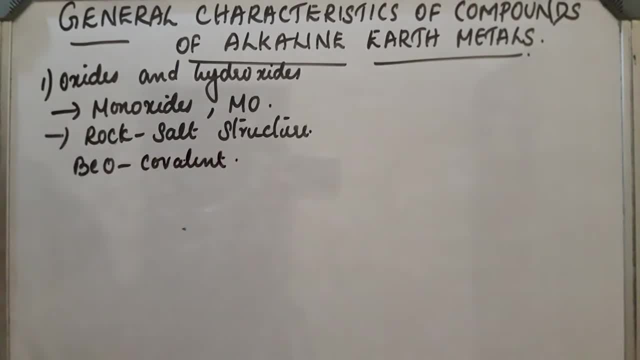 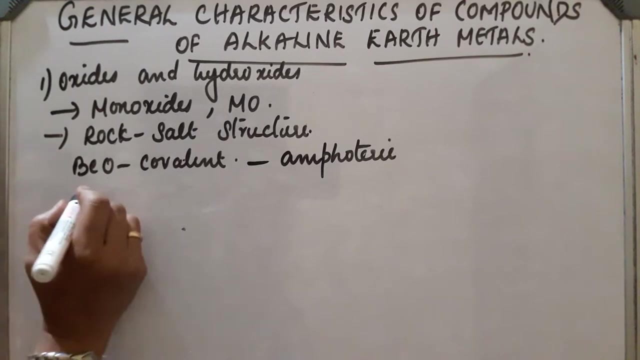 and enthalpy of formation of all the all these oxides are high and they are stable to heat. okay. beryllium oxide is also amphotric in nature, both acidic and basic. okay, but in the case of other oxides these are ionic, other oxides are: 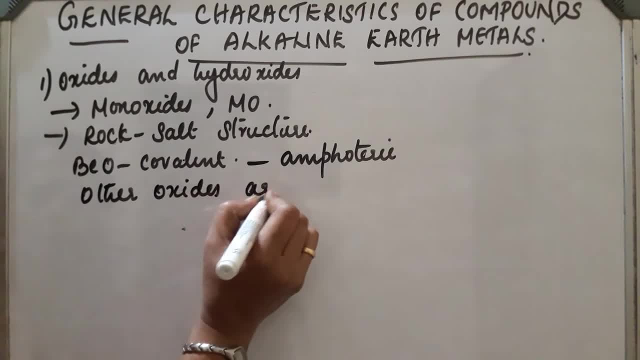 ionic, ionic, ionic, ionic ionic and their base city increases down the group and their base city increases down the group. so basic nature increases down the group there. all the others are basic okay. they react with water and form sparingly soluble hydroxide. 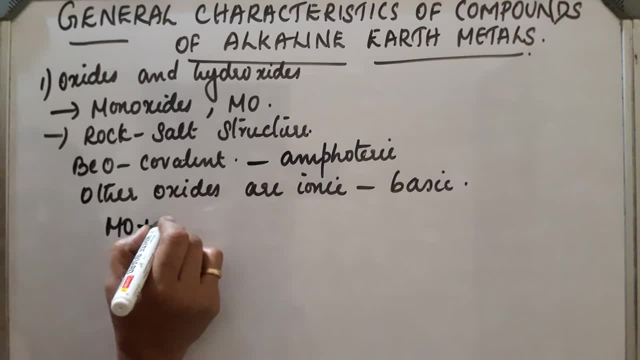 they react with water oxides. react with water means metal. metal. these metal oxides reacts with water and sparingly soluble metal hydroxides, and their solubility, thermal stability and basic nature of these hydroxides increases down the group. okay, Thermal stability, then basic nature. 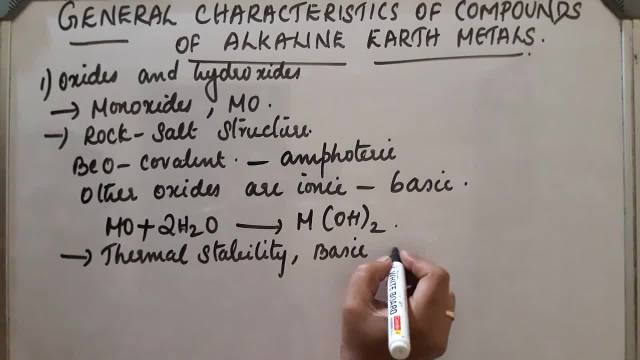 and solubility also increases down. okay, in the case of hydroxides. Next, compared to alkali metal, they are less stable and less basic, okay. And beryllium hydroxide is amphoteric, that is, it reacts with both acids and bases. With bases it form. 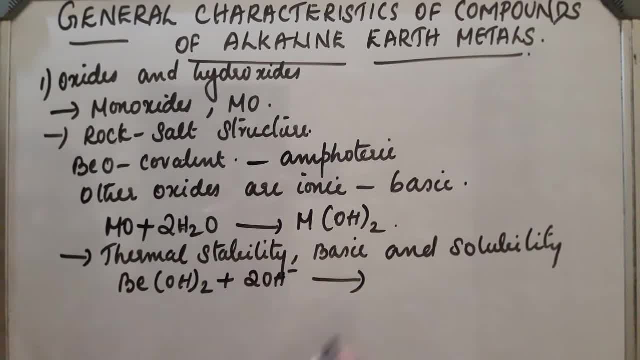 beryllate ion, that is, BE OH 4 times 2 minus okay. And with acid HCl, HCl plus 2H2O, it forms an hydrated compound: H2O 4 times Cl2.. This compound is: 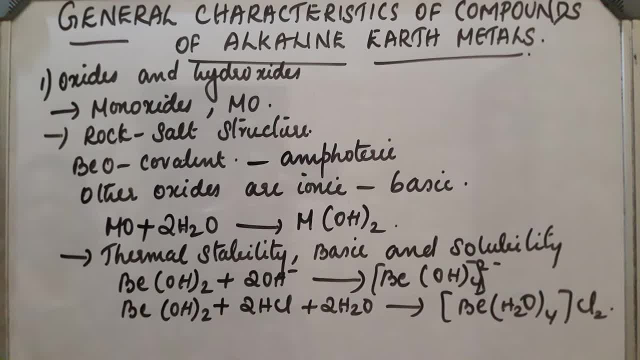 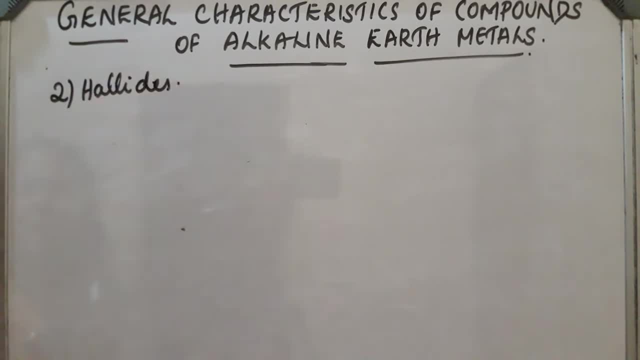 OH, Okay, next compounds: halides, second type halides. So beryllium halide is covalent in nature and all the others are ionic halides, that is, BEX2, which is also soluble in organic. 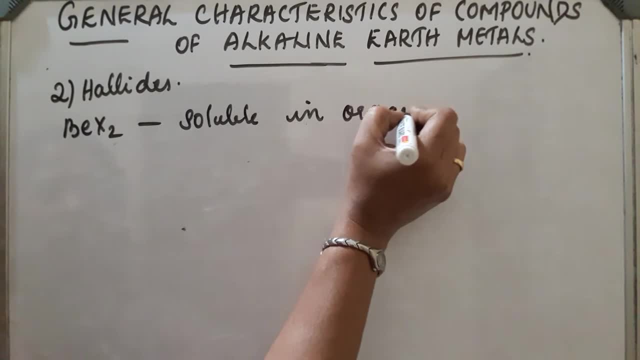 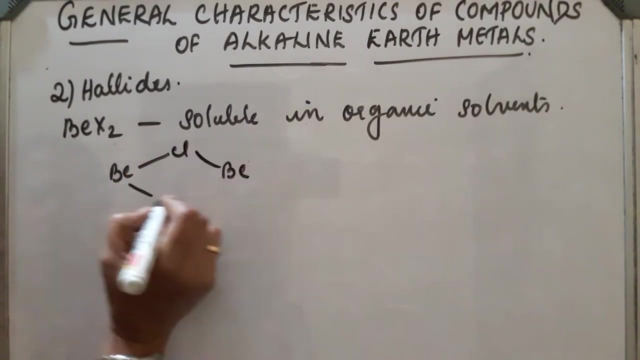 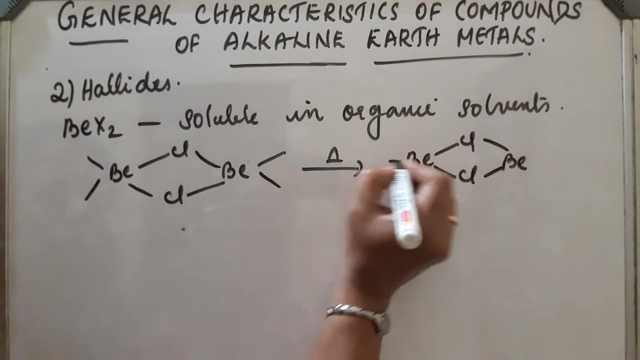 solvents okay. in organic solvents Okay, and B is here to form a chain structure. It forms a chain structure like this: okay. On heating. it forms like this: okay Again, on heating at 1200 Kelvin. 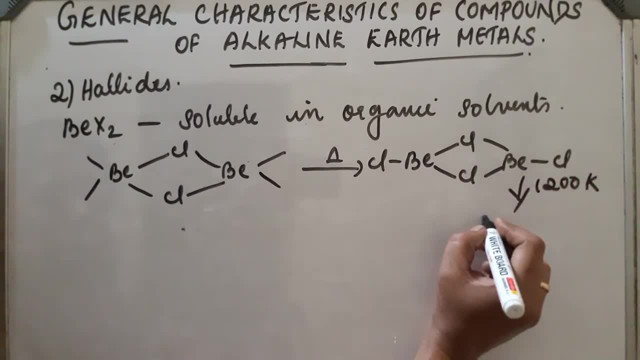 1200 Kelvin it forms a linear compound, BECL2, linear compound is obtained. So in vapor phase BECL2 form bridge dimer, okay, And at a temperature of about 1200 Kelvin, okay, 1200 Kelvin, it forms. 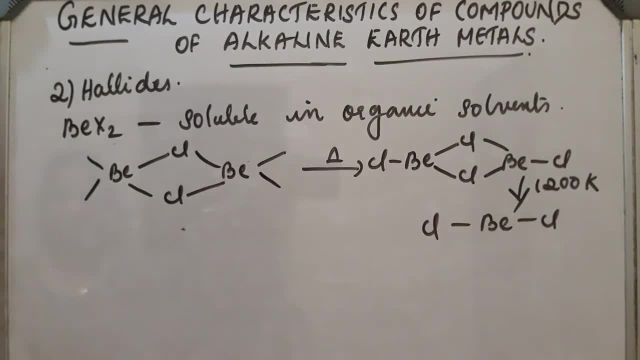 a linear compound. okay. And next, tendency to form hydrates: H2O: 3.5 times vaccinates. H2O decrease down, down. okay, It all these chlorides are hydrated H2O, then H2O, they are hexa hydrated, but tendency to form hydration decreases down. okay, They are dehydrated: okay. These are dehydrated NaOH. они вытекают и Reese. 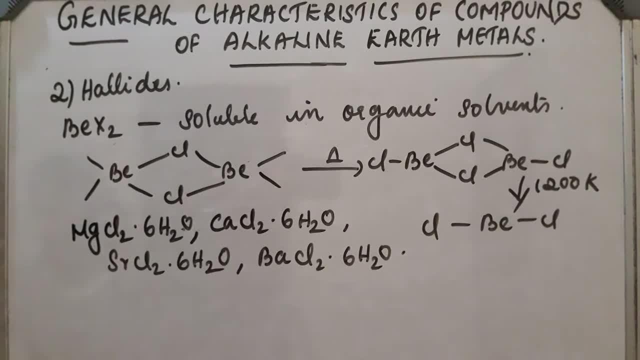 They are dehydrated, but tendency to form hydration decreases down. okay, application of H2O3 бер kingship amitak sentinels decrease down. okay, They are dehydrated. It is aầnอιODOSAT Mass gold less than more than 120. 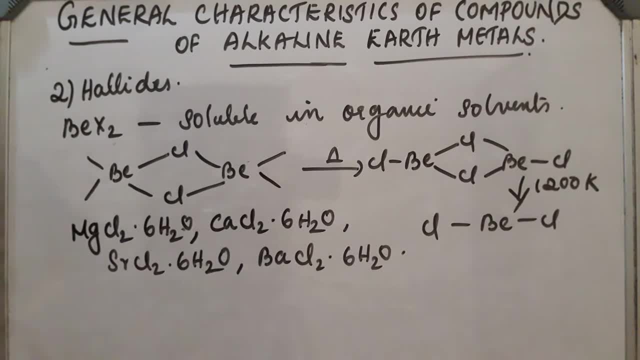 It is aussianat dihydrates than meterol, olderci plupart harmful to water. ok, They are dehydrated by heating. okay, all these chlorides, bromides and iodides of corresponding beryllium and magnesium, their halides, that is, their chlorides, bromides and. 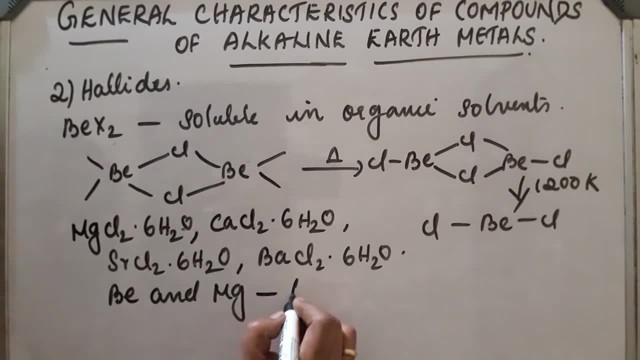 iodides on heating undergo this undergo hydrolysis. okay, this undergo hydro hydrolysis. but in the case of other compounds, they dehydrated on hydro heating, okay. next, what will happen in the case of fluorides, fluorides- fluoride is having smaller size, okay, so they are having high. fluorides are having high. 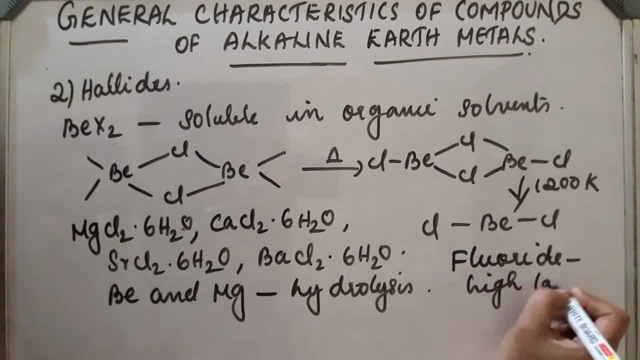 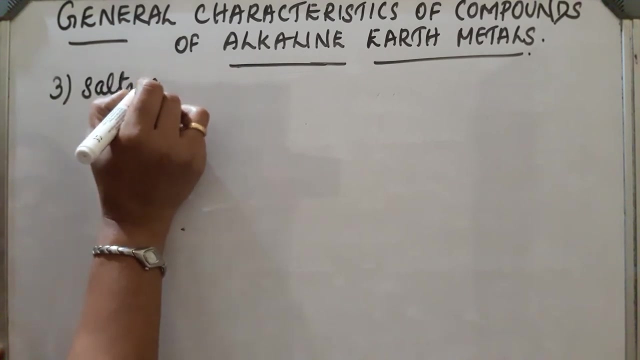 lattice enthalpy, so they are less soluble in water. okay, okay, so they are less soluble in water. okay, due to their high lattice enthalpy, they are less soluble, okay. next, third type of compounds: source of oxo acids. so third combo: source of oxo acids. so these 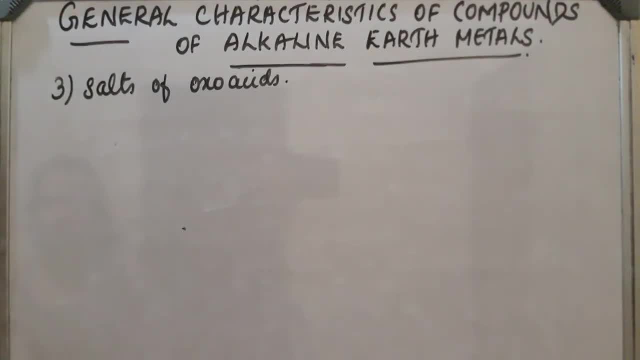 compounds this alkaline earth metals from source of oxo acids. they are carbonate, sulfates and nitrates. so third combo, Musso ali ess, would have the best result. Oooh, so for those of you who think of carbonate phosphorus, we just use one. 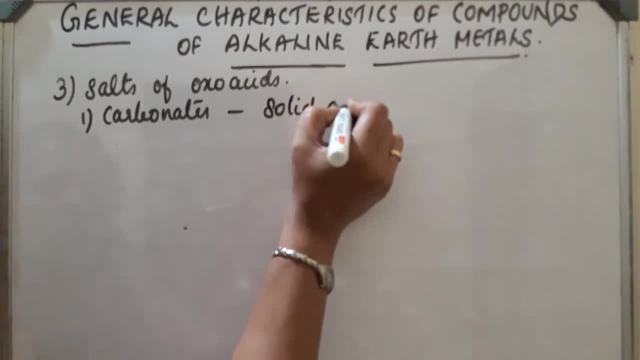 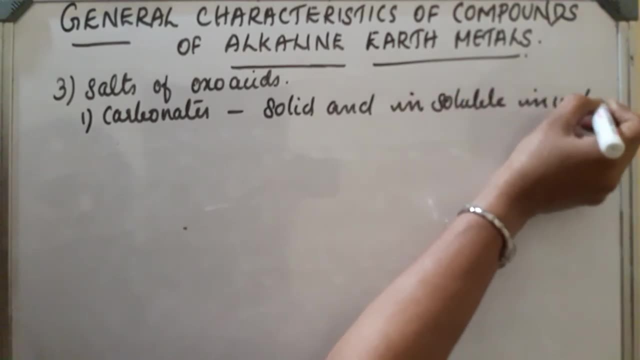 bit of a citric acid in the second combo. Okay, so this is some of the three carbons, right? so these are some Bื้ر 번 unserem the aspire. first one: carbonates. carbonates are solid Soled and insoluble in water. insoluble in water, okay, and they are precipitated. 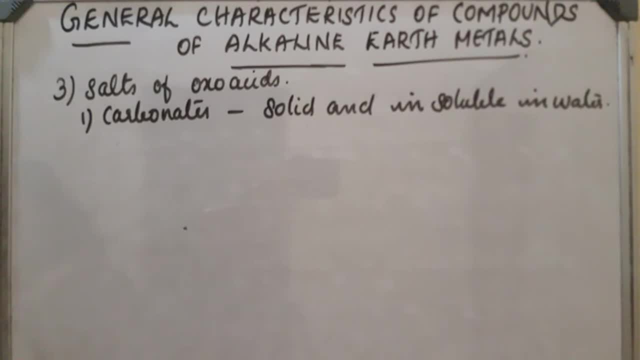 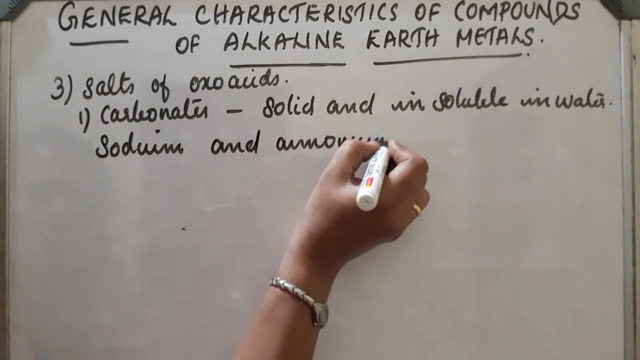 are soluble in water: okay, and they are precipitated. solution of a soluble salt of these metals: okay, the soluble source of this metal: we are adding sodium and ammonium carbonate, so they get precipitated. okay, ammonium carbonate is added to the soluble salts of these metals. they get precipitated and the solubility of 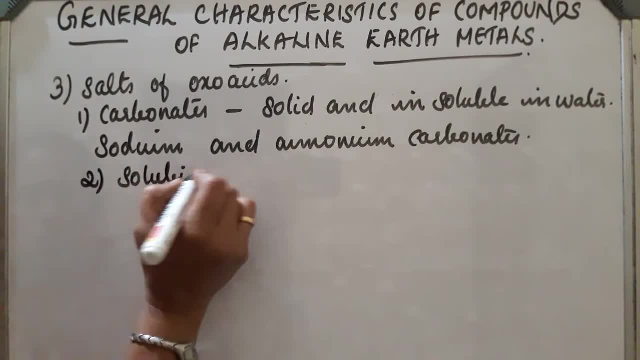 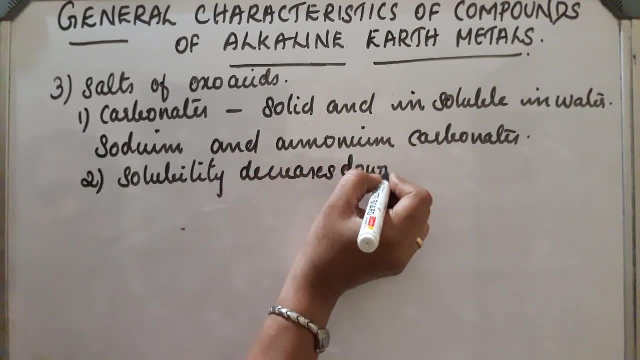 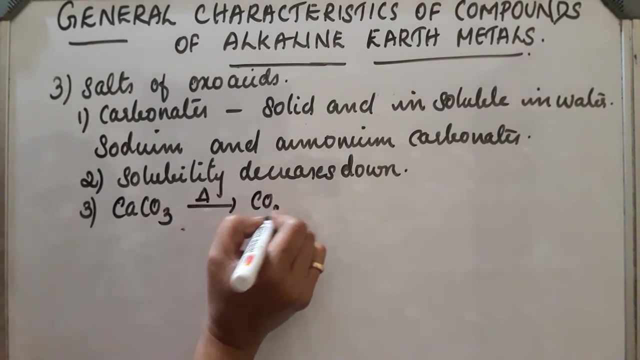 carbonates decreases down. solubility decreases down. decreases down the group okay. next, on heating, this carbonate decomposes and form carbon dioxide and metal oxide, for example ca co3. on heating gets decomposes to carbon dioxide and calcium oxide and the temperature of decomposition increases from magnesium to beryllium. so temperature increases from down the group okay. but in the 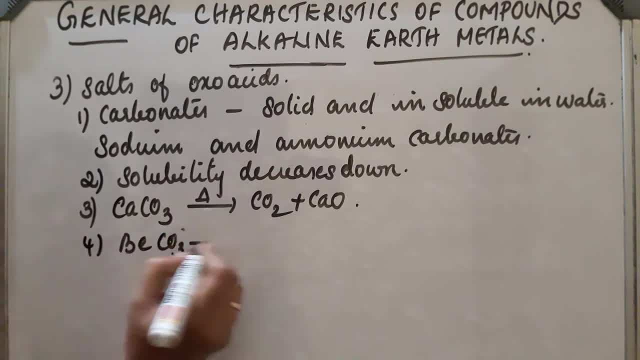 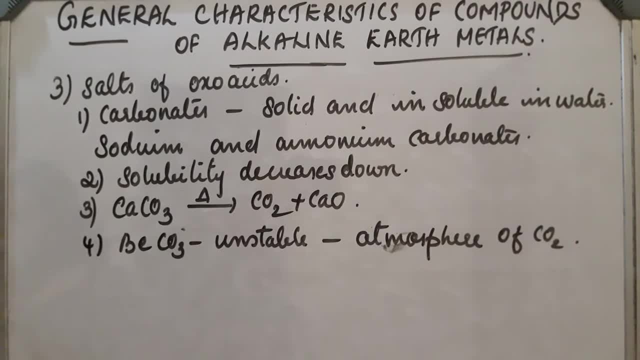 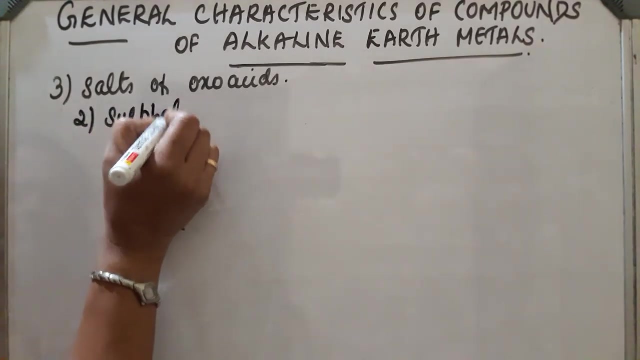 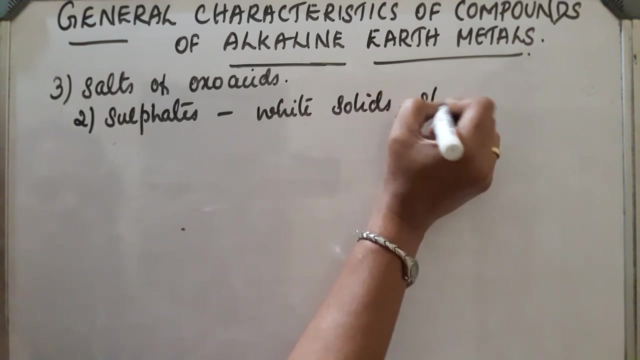 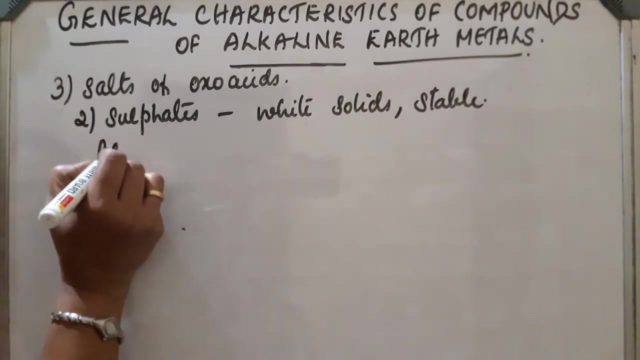 thermal stability increases down as the cationic size increases. okay, thermal stability increases down the group. thermal stability increases down the group. so second type of salt is sulfates. so sulfates, they are wide solids and they are stable to heat. okay, now in the case of beryllium sulphate and 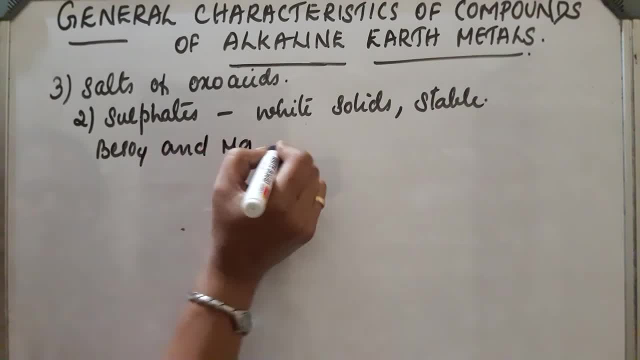 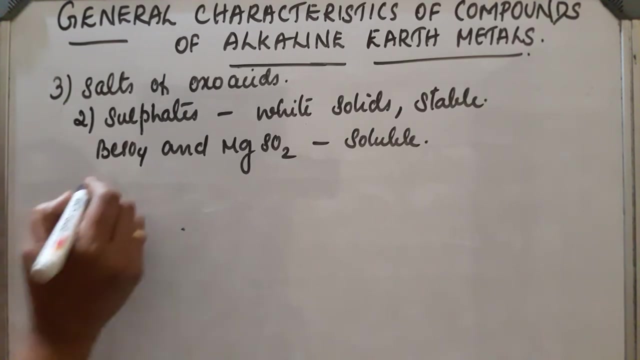 magnesium sulfate. theirjack s soluble in water. They are readily soluble in water because of their smaller size and high hydration enthalpy. They overcome their lattice enthalpy and they are easily soluble in water, but the solubility decreases down. solubility decreases down. the group. 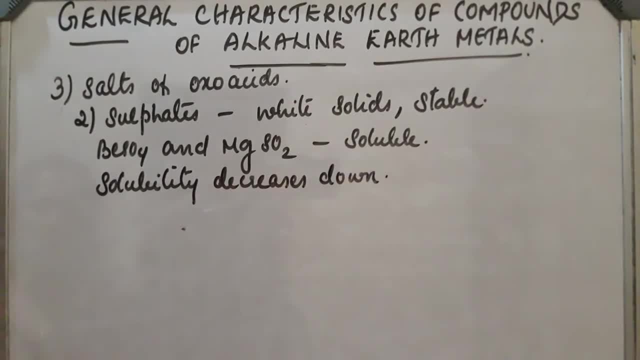 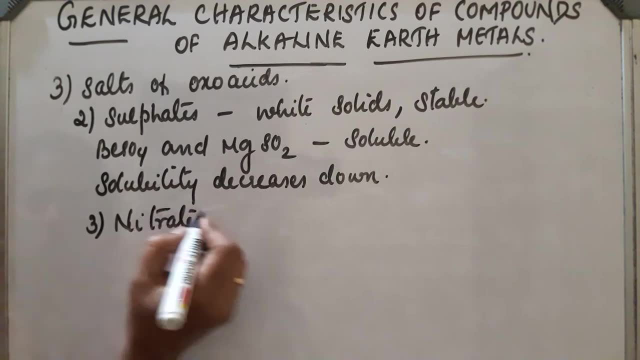 As the size increases, solubility decreases. Next, next type is nitrates. What about nitrates? Nitrates are made by the dissolution of carbonates with dilute nitric acid. They are obtained by dissolution of carbonates.